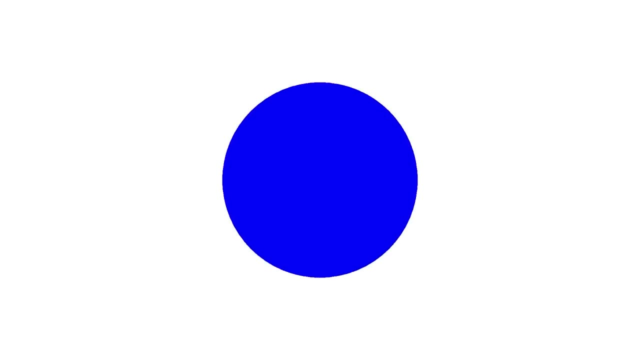 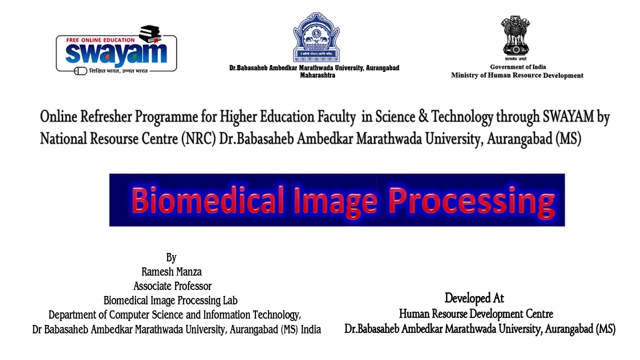 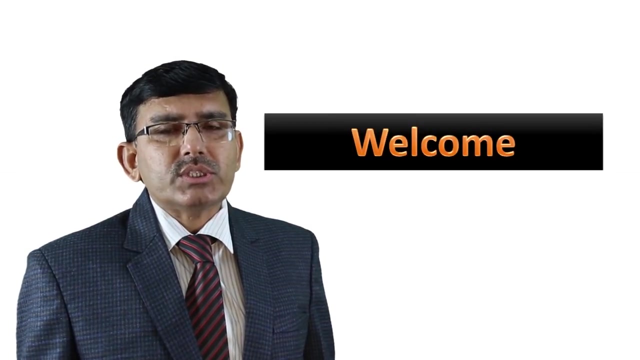 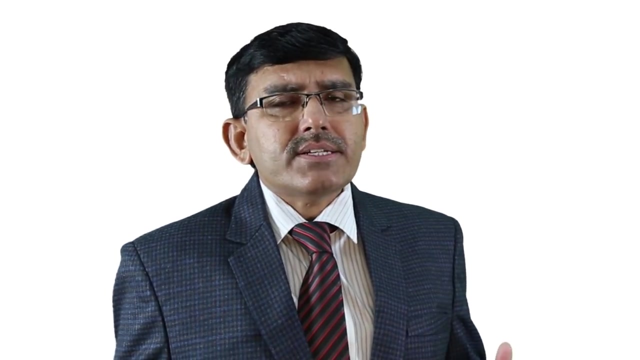 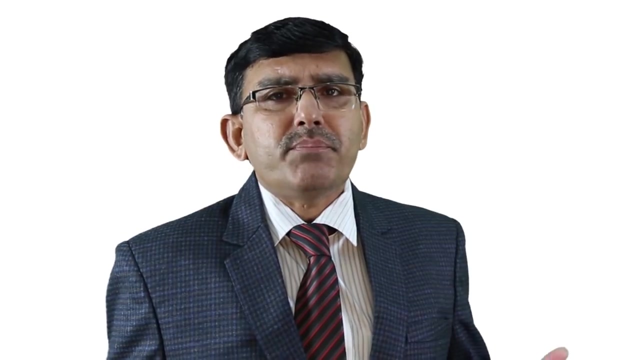 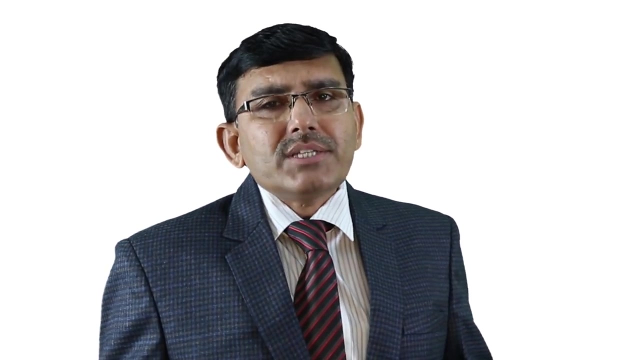 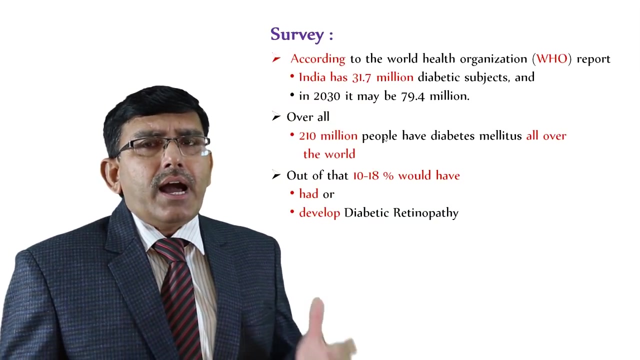 Welcome to biomedical image processing course. This course is important for the researchers, academicians and industry professionals to learn how to diagnose the diseases and how to make the treatment for the patients. Through this course, our objective is to make system automated so that patients can able to save their life. According to world health organization, in India, around 31.7 million patients are suffering with diabetics and it will reach to 79.4 million up to 2030.. Overall, worldwide 210 million patients are suffering with diabetics, whose growth rate is 10 to 18 percent for the forecast years. We have tremendous opportunities. 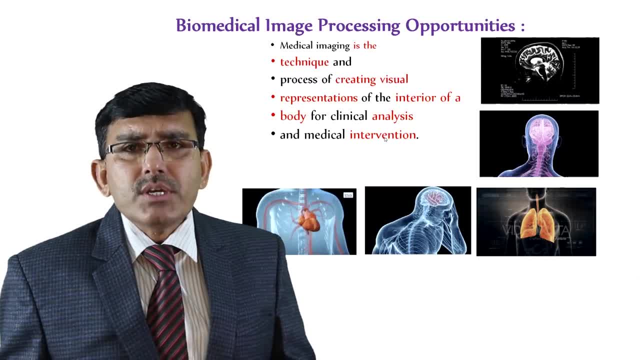 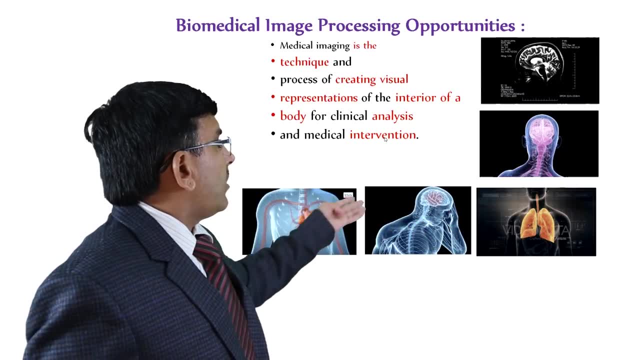 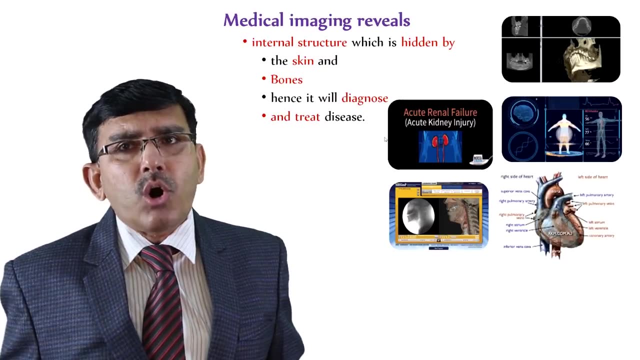 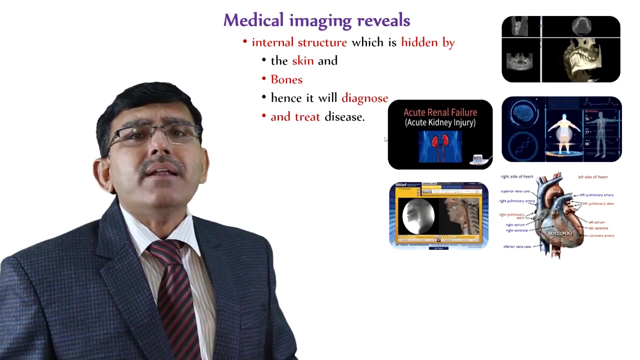 using biomedical image processing, because we can able to diagnose the inner part of the human body and decide the effect of diseases on their organs, How to plan for the process of their treatment, and so on. Here our objective is to get the inner portion of the human body and make the treatment plan for them. 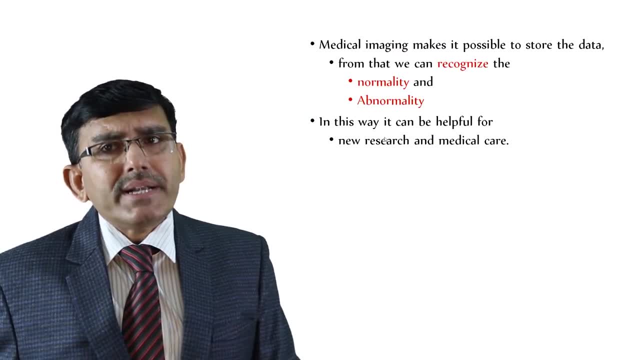 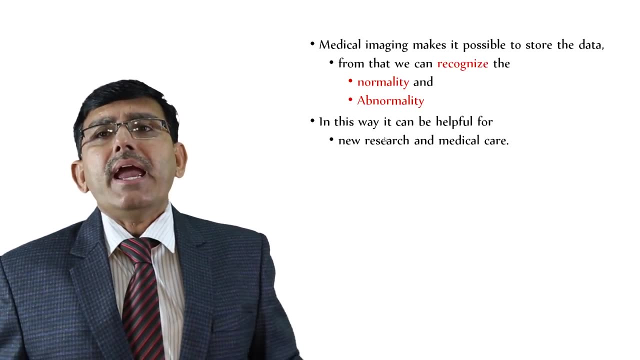 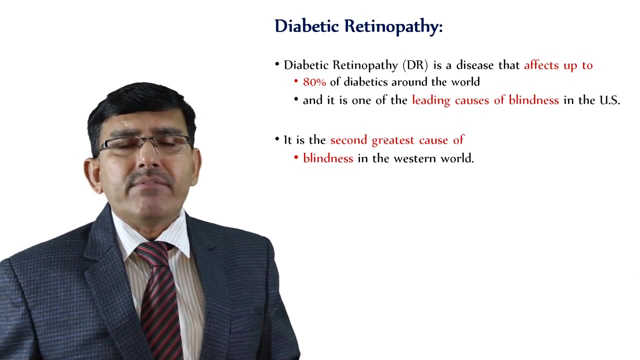 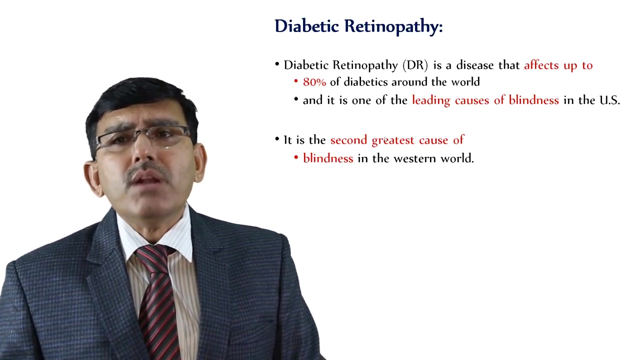 To make the process automated in such a way that it will do the classification either of normality or abnormality and hence researcher can able to learn how to make these classification effective. Diabetic retinopathy has the patients suffering around 80% worldwide and it is the major cause of blindness for the people which are living worldwide. 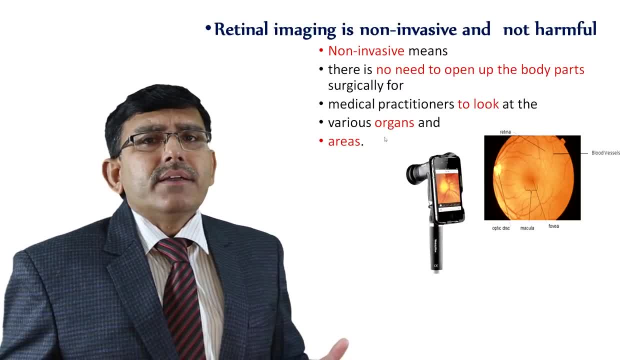 And hence this is non invasive technique because we can able to capture the retinal image using a simple cameras, And that's why it will not affect on anyone living there. We can use the simple cameras to capture the detailed image of the patient. Without the use of micro cams, we can capture the clinical image from the patient. 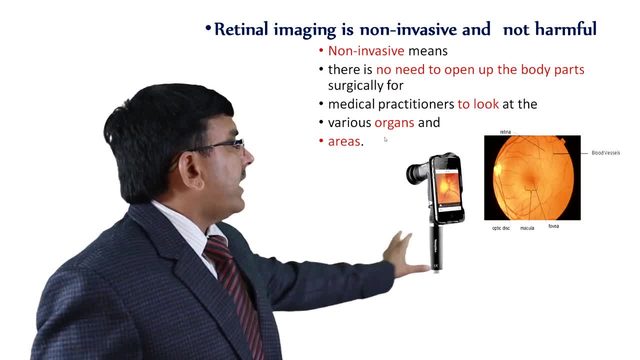 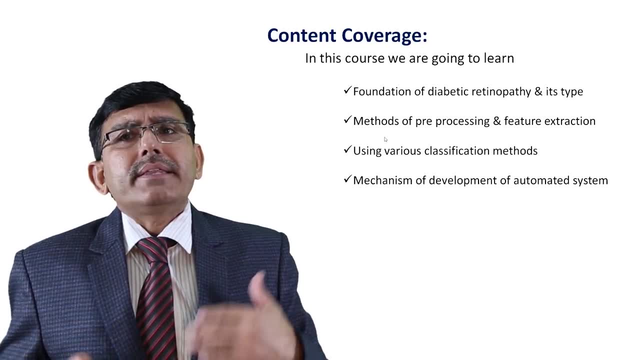 Without the use of micro cams we can not capture the clinical image from the patient, So it is a very simple technique. This is the basic technique we can able to use in healthy people, any part of the body. here we will cover the diabetic retinopathy, its different types. 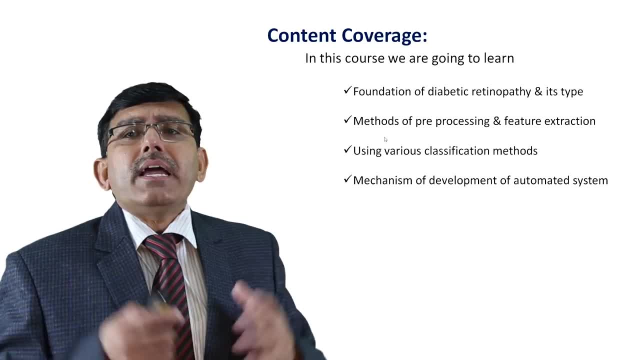 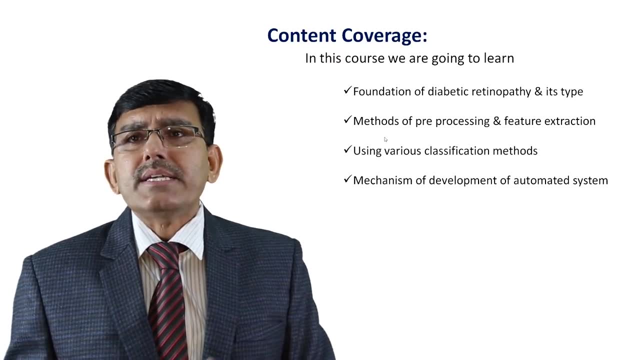 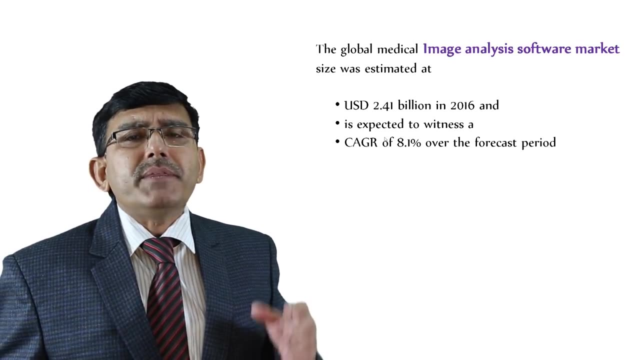 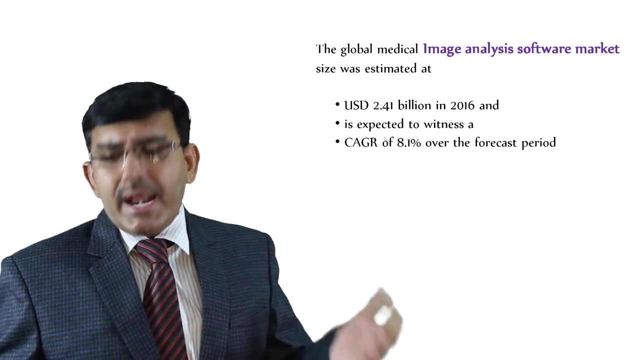 pre-processing technique, feature extraction technique, classification technique of the images and make the system automated for the process of diagnosis is the major coverage of this particular course. diabetic retinopathy is one of the condition through which the inner wall of the neuro vein are thick, hence fluid cannot be flow and hence patients started to be suffer with. 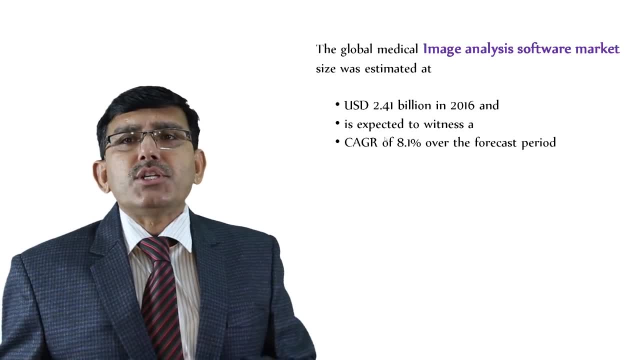 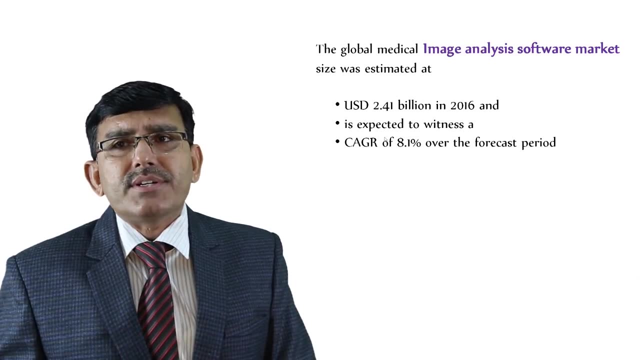 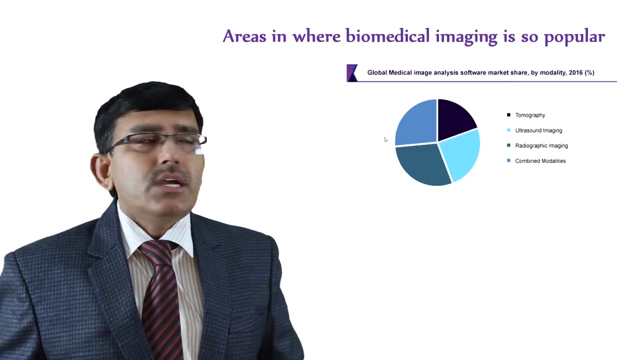 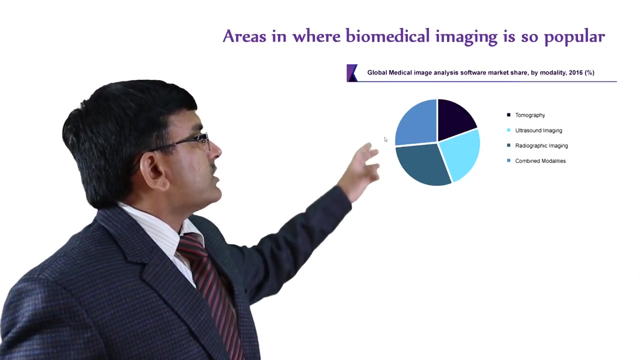 diabetic retinopathy image analysis, which is used as one of the software having contribution 2.41 billion in 2016 and it will reach to 8.1 percent growth rate for the casting years. we have other different modalities, like mri, ct scan, x-rays and so on, to diagnose a. 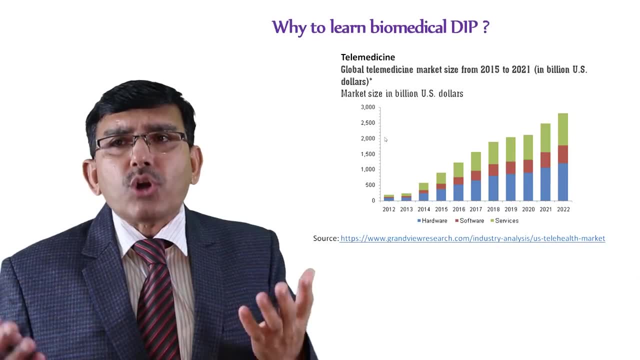 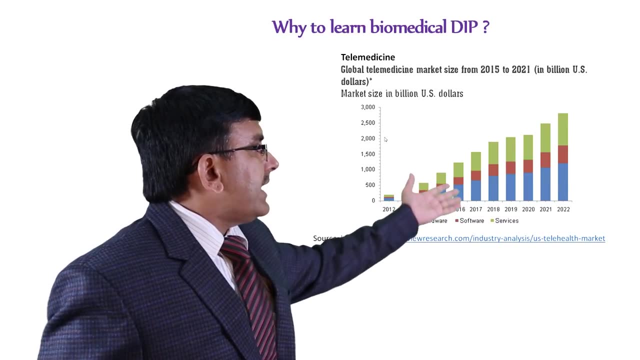 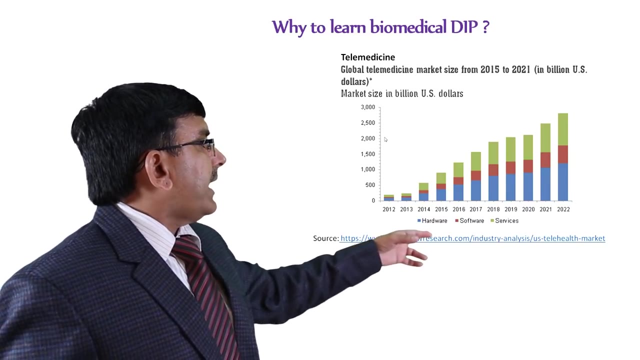 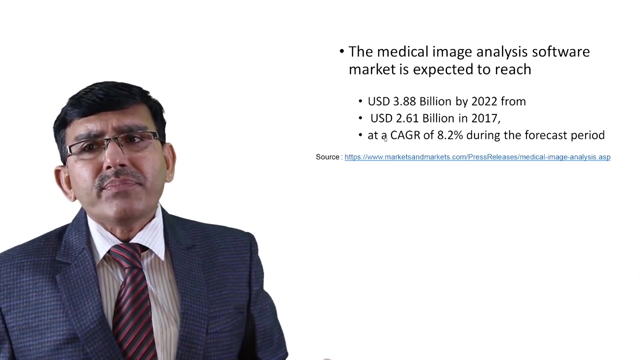 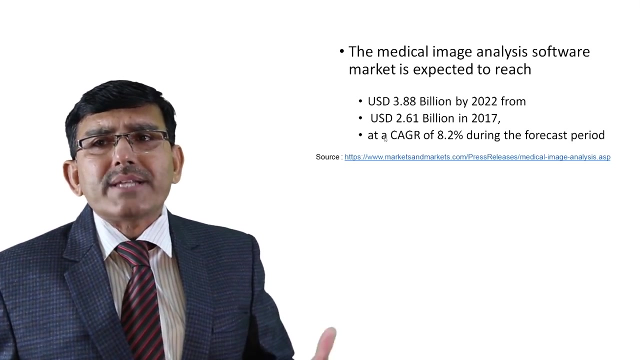 particular diseases. sometime we can use combination of multiple modalities so that it is possible to diagnose the disease which are hidden in other modalities too. this graph shows that how much amount of the contribution done by image analysis software worldwide. in 2017 it was 2.61 billion. in 2022 it will be 3.88 billions. the growth rate is 8.2 percent for the. 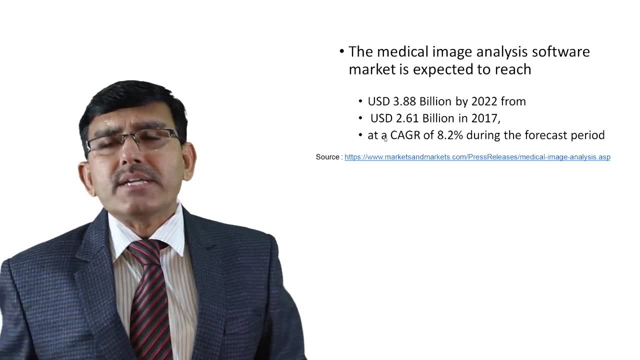 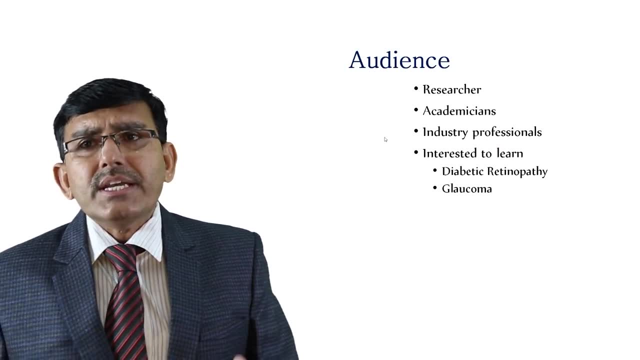 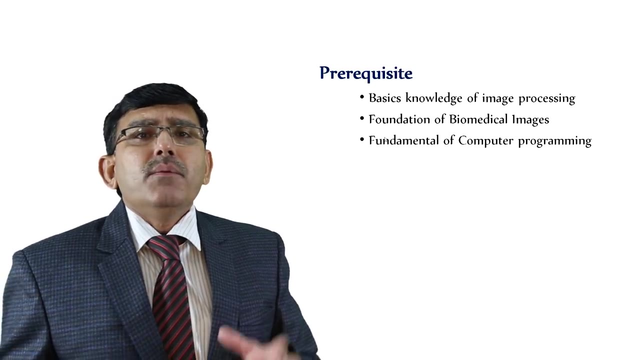 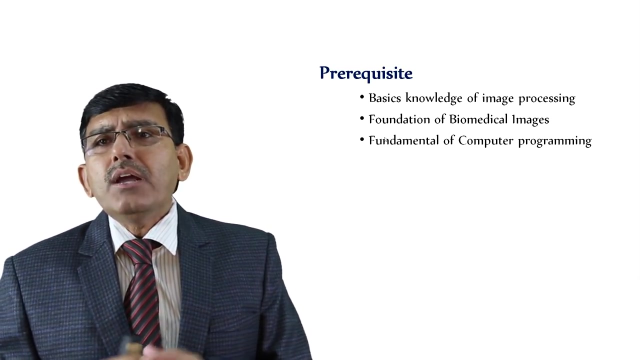 further forecasting years. it has shows the importance of this particular area. the expected audience for this course are researchers, academicians, industry professionals and all the researchers which are working in biomedical image processing. prerequisite expected are basic knowledge of image processing, foundation of medical imaging, fundamental knowledge of 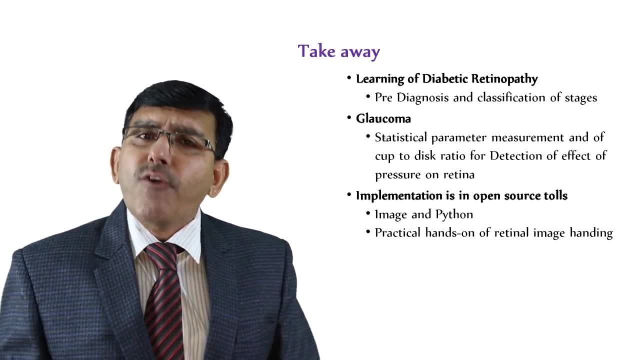 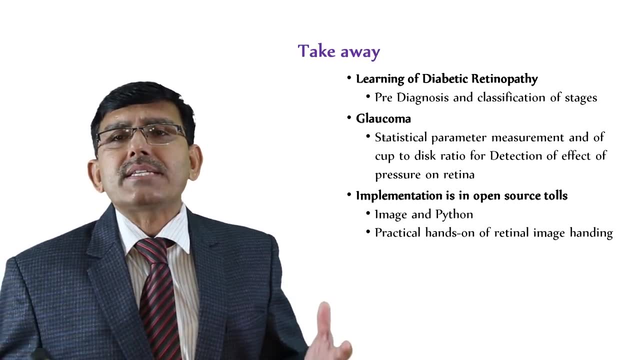 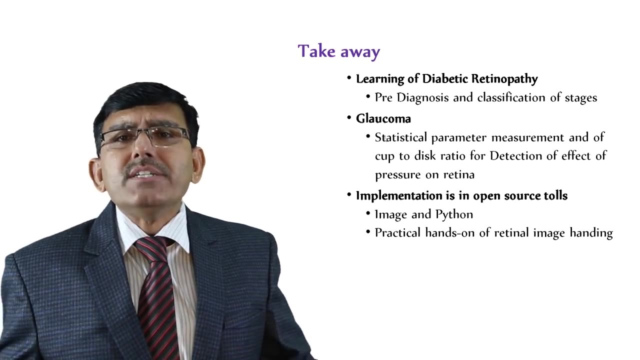 programming languages, etc. the takeaway for the audience from this course are how to do pre-diagnosis classification of the disease, like diabetic retinopathy, glaucoma and so on. all the modalities we will implement with hands-on training through open source software like python. so i request you. to please join this course, thank you.